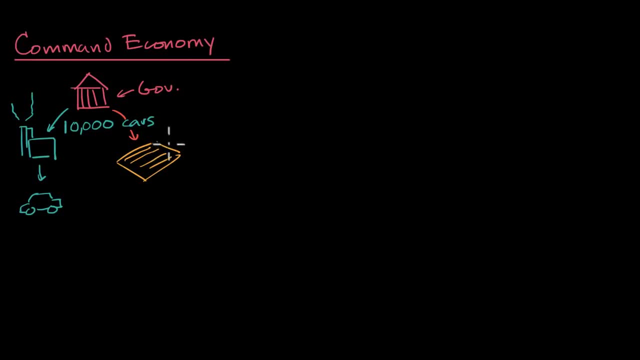 And this is my best drawing of a field really fast- And so it needs to say: hey, you need to produce- I don't know- 10 million apples. I don't even know if that's a reasonable amount of apples to produce. 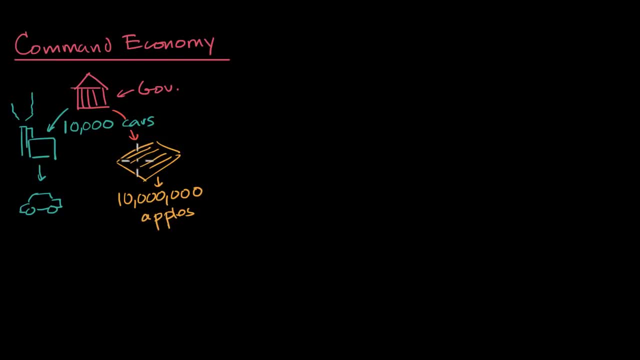 But you need to produce 10 million apples, and so the farmers who essentially work for the government, because the government would own that farm- they would produce those apples. And also in a command economy there's like: well, who gets these cars and who gets these apples? Well, in an extreme command economy, they will be directly allocated by the government. The government will say: all right, you get a car, you get a car, you get a car. It will not be based and in fact it will not likely. 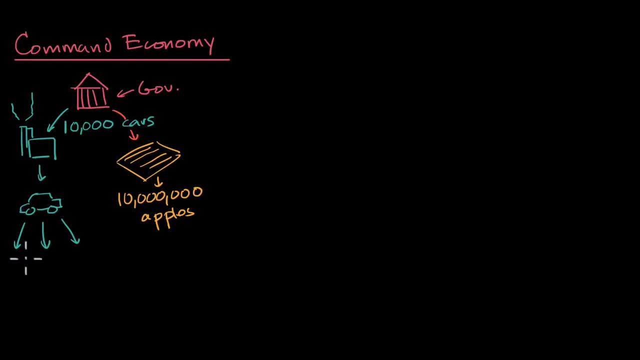 be based on any type of who's willing to pay for the car or who could pay the most for the car. Similarly for the apples. So they're all going to be allocated. So there would have to be a lot of planning done on the part of the government to say okay. 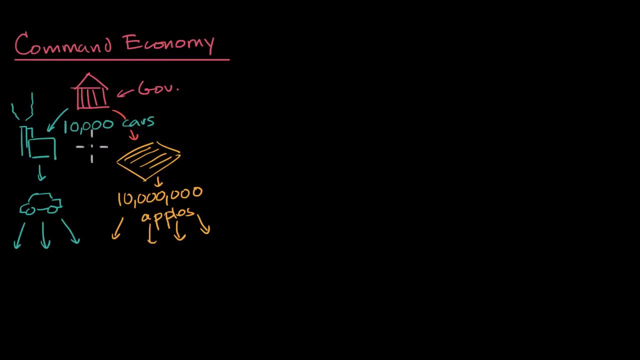 how much should we produce of one thing versus another thing, And how do we decide who gets the different things? Now, the other side of the spectrum. you have what's known as a market economy And most economies in the world, especially the United States. 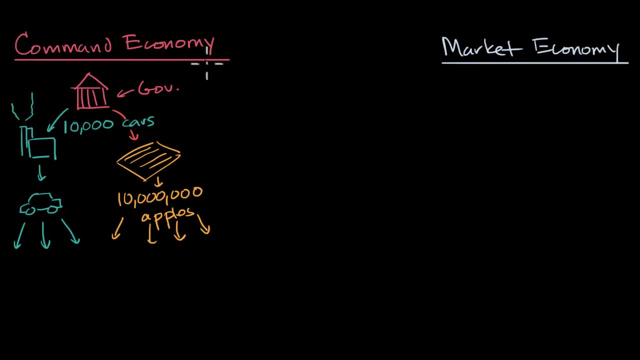 are much closer to being a market economy than being a command economy. Rather than having the government owning the factors of production, deciding who produces what and how much and who gets those things, in a market economy it's all based on the factory. 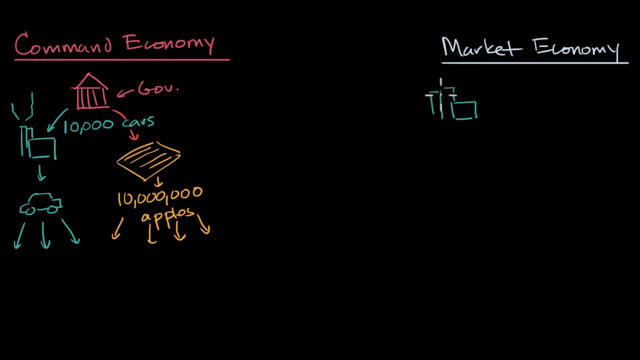 right over here- independent of the government for the most part, unless you're in certain fields that might have strong influence from the government. Let's say you're a military contractor. But if you're not in one of those fields, you're fairly independent of the government. 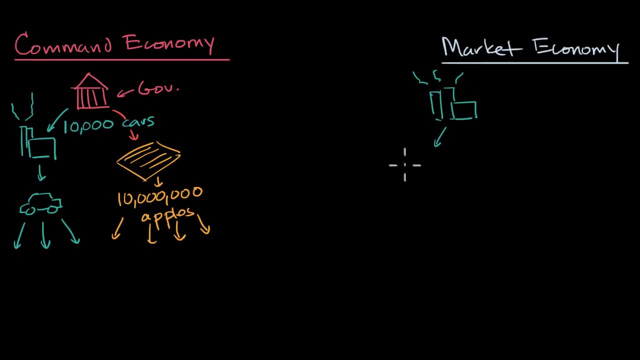 what they would say is: well, what does the market need? They might say: hey look, the market needs 5,000 cars that look like this, but then it also needs another 2,000 trucks that look like that. 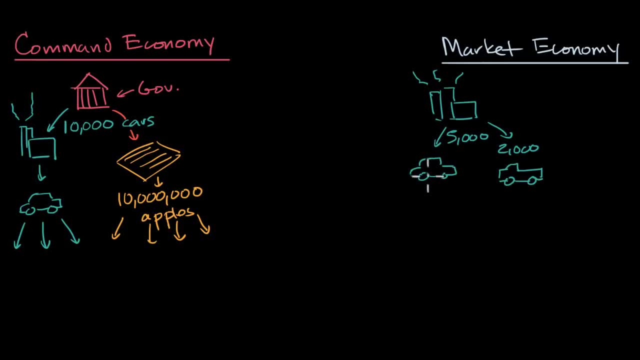 And how are they basing it? Well, they might have looked in the past year. well, how well is this car selling, How well is the truck selling? They might look at competitors. In fact, in a market economy, you'll often have more competition. 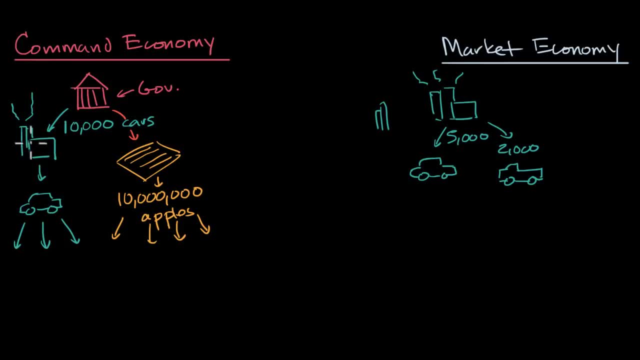 In the command economies you might have one really ginormous factory that's owned by the government, or a few, while here you might have competing factories where they're always: hey, they make a pretty good car, we're gonna make one that's just as good. 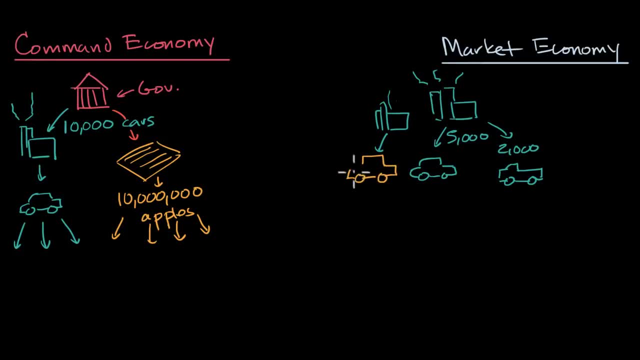 and it comes in yellow. So once again you have this notion of competition for people to produce things out in the market, and they're also making their best judgment of what does the market actually need. Similarly, you could have your farmers here. 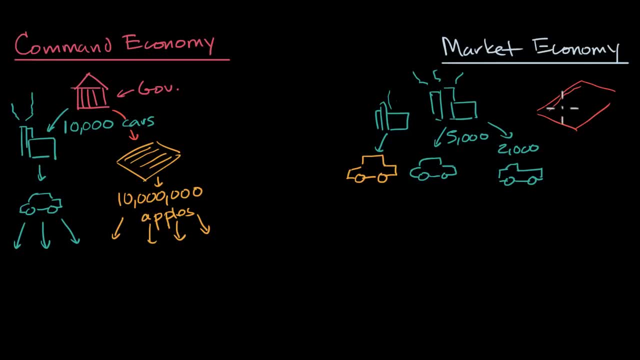 and you say: hey, you know what? I've been growing a lot of apples, but that doesn't seem to be in demand anymore, so I'm going to grow more. I don't know peaches, because it looks like the sale of peaches. the peaches are in fashion this year. 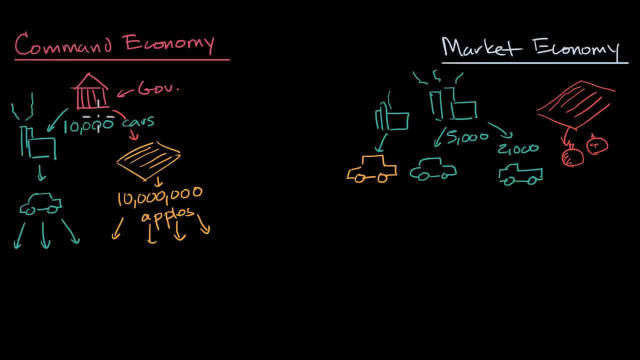 And similarly, who gets these is not dictated by the government, it's determined by the market. And so let's say this is me, let's say this is you, let's say this is someone else, If I might not be interested in getting a truck. 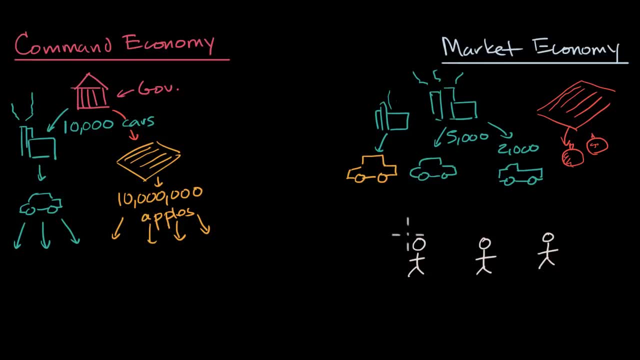 but I really need to get a new car for my family so I can drive them around and take vacations and things. and let's say you want to get a car too, but the market will dictate who gets it, So, for example, the factory might set a price for this car. 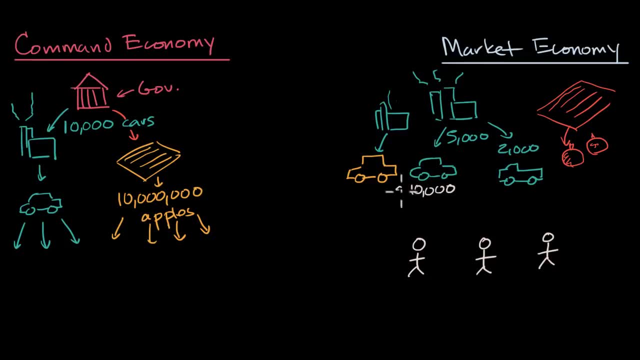 They might say: it is $10,000 per car And maybe I'm willing to pay it, maybe I'm not, Maybe I'm just like: well, I really like that blue car, but I'm not willing to pay $10,000,. 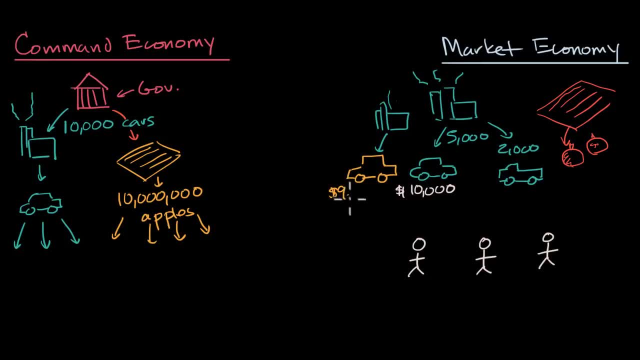 and this yellow car is available for $9,000, so I am going to get that, And the prices themselves won't necessarily be fixed. If they're not selling enough of these cars at $10,000, they might lower the price. 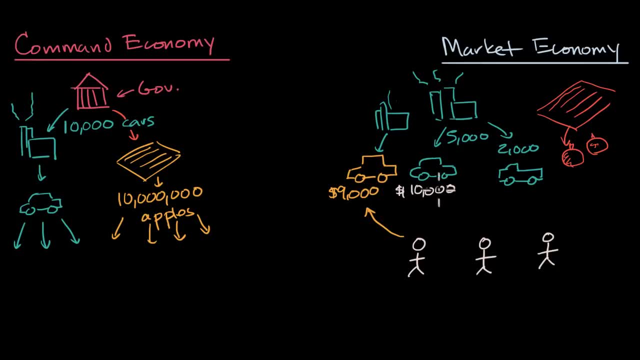 to compete with the yellow car at $9,000.. Similarly, if there's a ton of people who are willing to pay the price of this truck, they might raise the price on that truck or produce more of it. And the severe competition if one firm doesn't do this well. 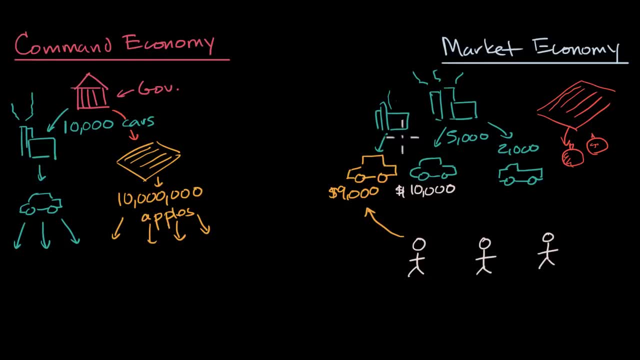 on a regular basis, they might go out of business. So there's a strong motivation to be able to meet the needs of the market, and then the prices adjust accordingly, And so you might say: well, what are the positives and negatives that people? 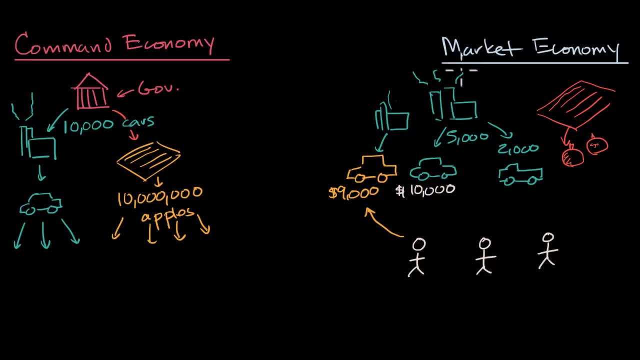 generally associate with command economies or market economies. Well, the motivation that's often given for a command economy is some notion of fairness or some notion of equality, That when you have a market economy as a byproduct of this mechanism where different people are competing, 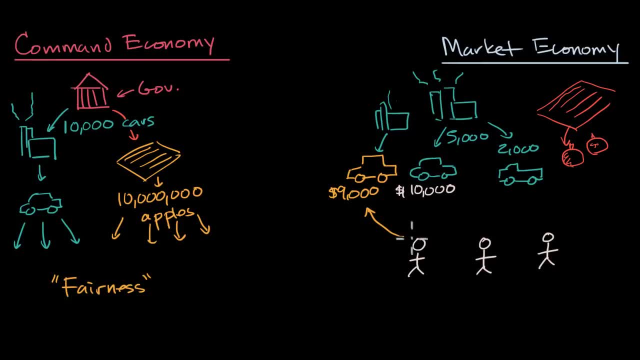 some people are innovating more or less, some people might be working harder or less, some people might just get luckier or unluckier. you naturally will have some level of inequality, And some of the original ideas behind command economies like communism were: hey, we don't like this inequality. 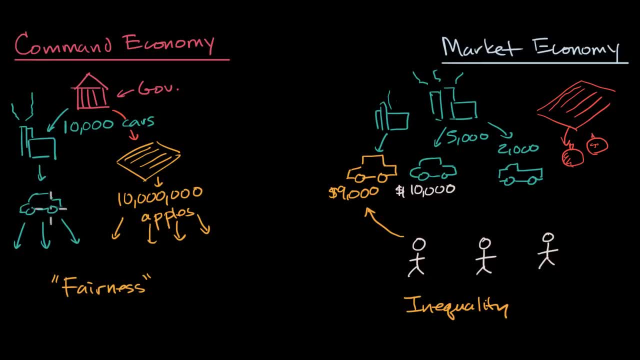 We want to see more fairness, And so we want to see everyone get exactly the same car. We want to see everyone get exactly the same number of apples. We don't want to see all of these competing firms. We want one really big, efficient factory. 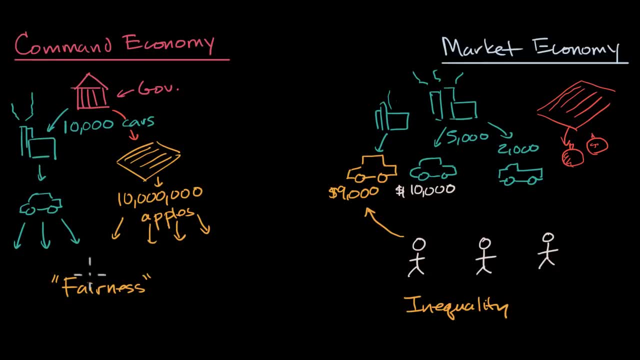 to just churn out these cars. Now it turns out in reality that's a little bit utopian. Even at the peak of some of these communist economies there were people who had better access to certain things, people who might have carried favor with the leadership. 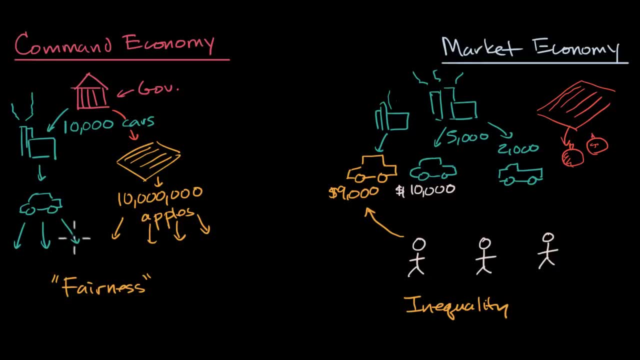 had more power, who had better apartments, had better cars, had more access to resources than people who didn't. In a market economy, yes, there will be some inequality, but the best thing going for it and the reason why most economies in the world. 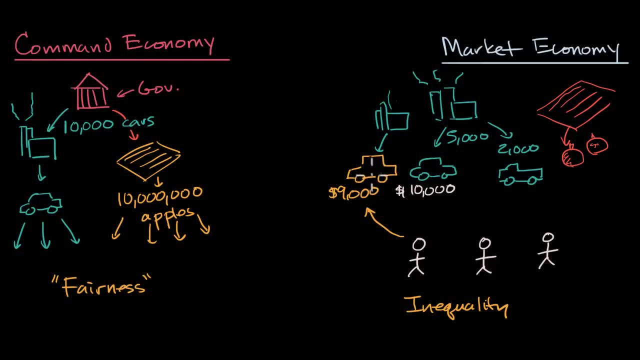 even ones that are nominally communist, like the Chinese economy, have traditionally been, have transitioned to a market economy, because a market economy is also associated with things like innovation and strong incentives for people to innovate or work or do things. Think about the situation in a command economy. 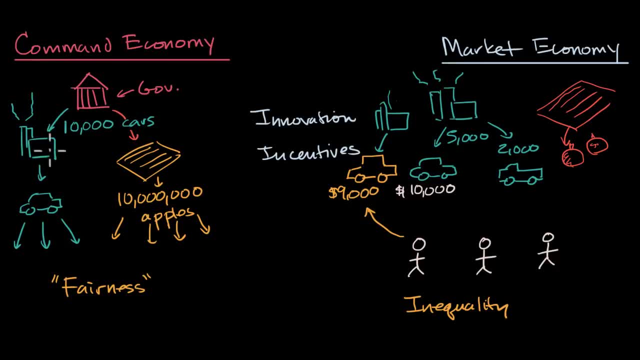 Let's say that you're a manager at this factory here. The government has told you to produce exactly 10,000 cars in exactly the type of model. Maybe you have an idea for how to make this car more efficient, but no one's really gonna reward you. 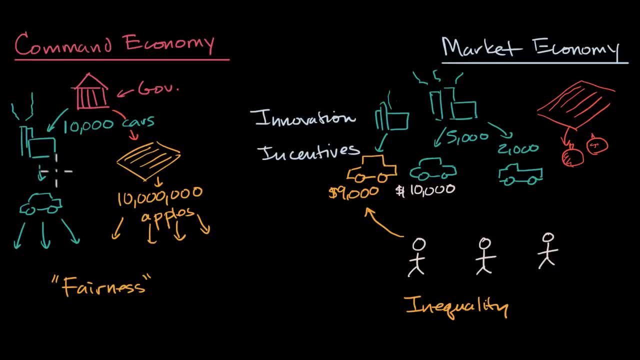 for that if you're not gonna be able to get paid more so that you can buy more things, You might not be as interested in doing it, While in this situation you have extreme competition where, as soon as this factory or this company is outselling this one, everyone here is gonna think: 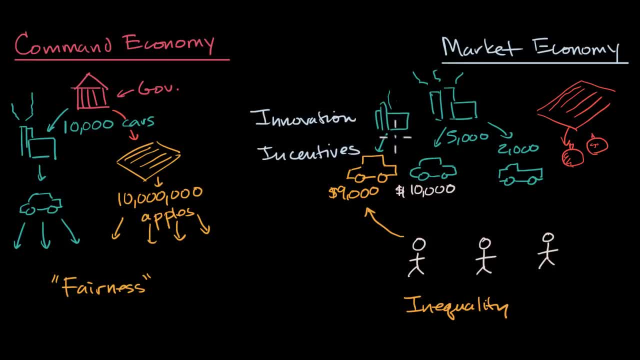 wow. we need to innovate, we need to really work harder so that we can take more market share from the other company. Similarly, at the individual level, different people might say, hey, I can only afford the yellow car now, but gee, I really wish I had the blue car.